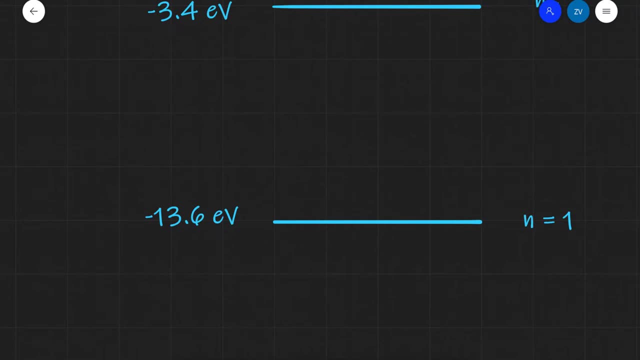 so here is where it gets really, really interesting. now imagine that you have an electron that's been excited to a higher energy level- and let's say that it is at minus 3.4 ev- and then it loses its energy and then goes down in energy level all the way down to the ground state. so if an electron 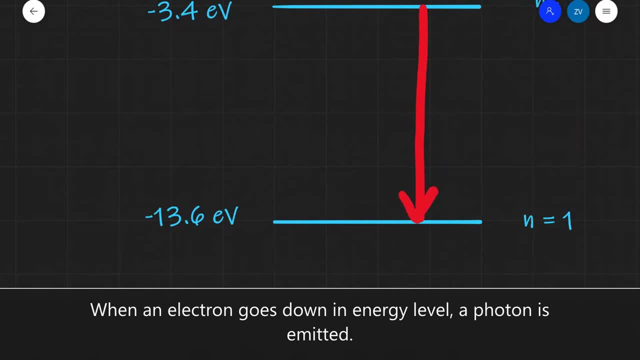 goes down in energy level. that energy has to go somewhere, and then a particle of energy goes down to the ground state and then it loses its energy and then it goes down to the light known as the photon is released. on the other hand, if we have an electron which is already in, 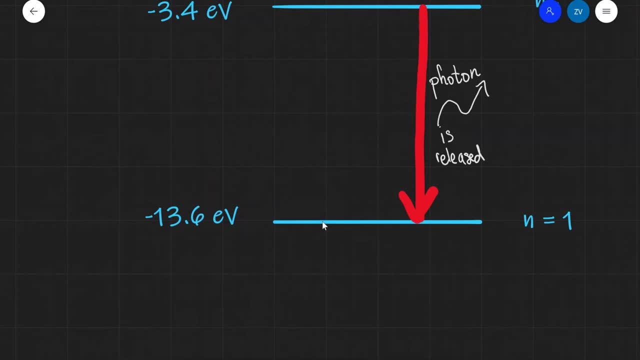 the ground state, it's at its lowest energy, and then we bombard that, that electron, with some photons. this electron could jump an energy level, so from minus 13.6 it will go up to minus 3.4 ev. so if that's the case, this is an indication that a photon has been absorbed. this is just pure energy. 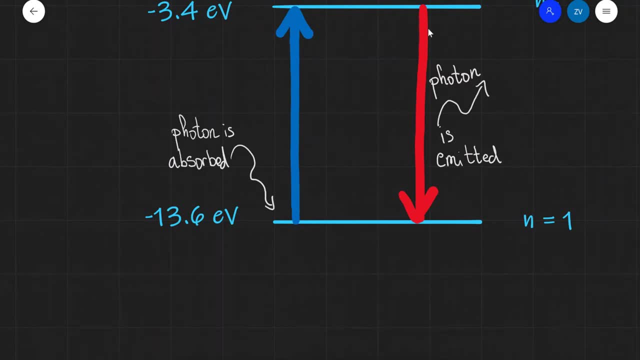 conservation. so in this case in which a photon is emitted, the electron will go down energy level. if it goes up in energy level, that means that that energy has arrived from somewhere. so a photon, a particle of light, must have been absorbed, because this is an indication that a photon has been 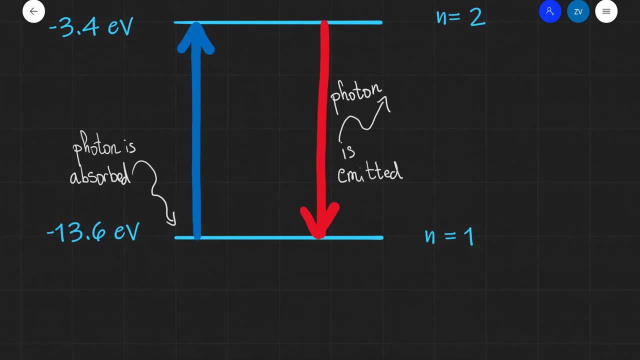 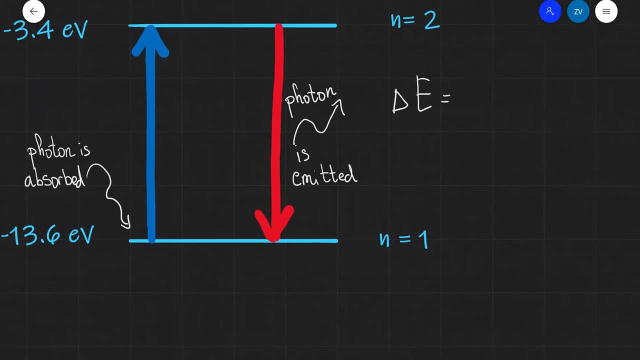 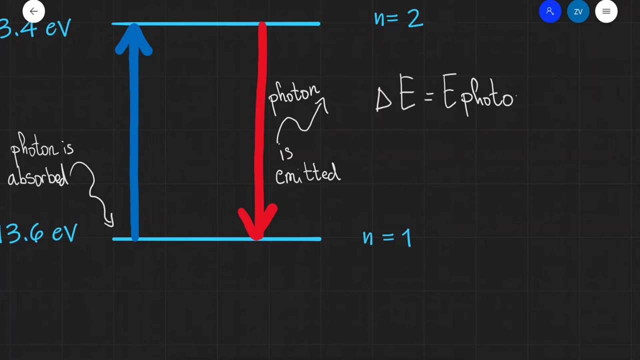 absorbed. this is energy conservation. in both of those cases, our change in energy- so we can write this as Delta E will be equal to the energy of the photon. so we can just say that this is equal to the energy of the photon. we know two formulae that are going to be useful in this case. 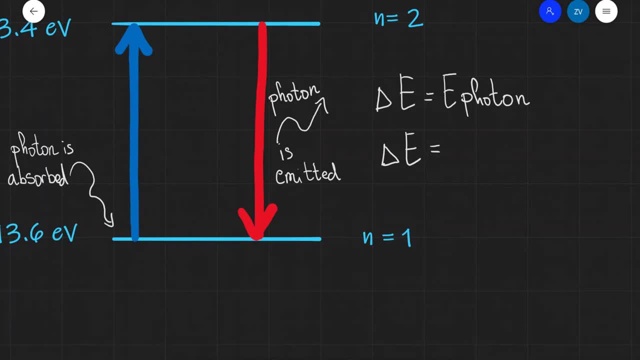 from our first year, quantum mechanics. we remember that delta, that the energy of photon isStop Mexican Virtual Computing Board, one of the ten most performing observantLevels of the Belt of Inspiration, either HF, or we could also write this as delta E is equal to HC over lambda, where